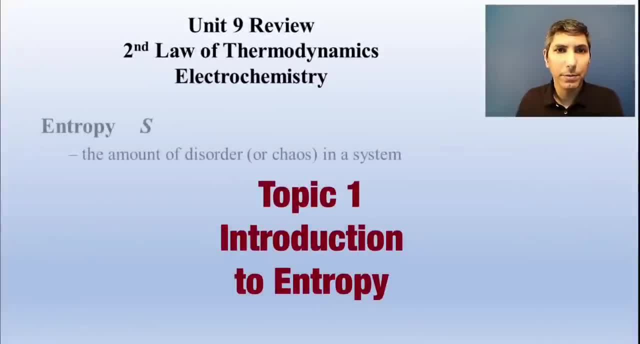 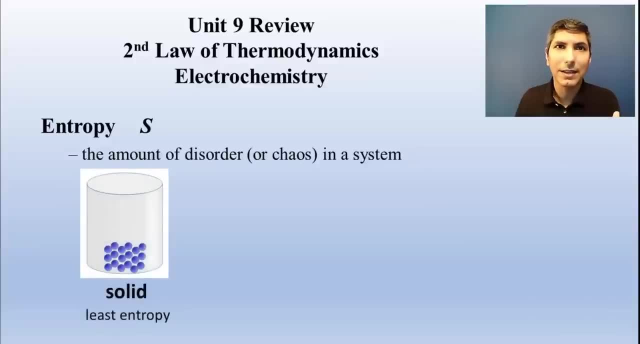 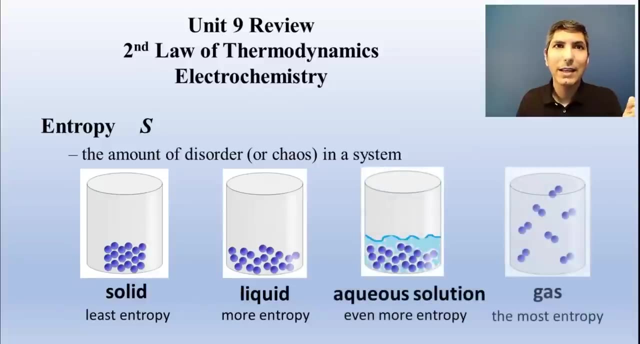 Let's get started. We often describe entropy as the chaos or disorder of the molecules in a system. Since solids have relatively little chaos, they have the lowest entropy, Liquids have more entropy, aqueous solutions have even more entropy and gases have the highest entropy. 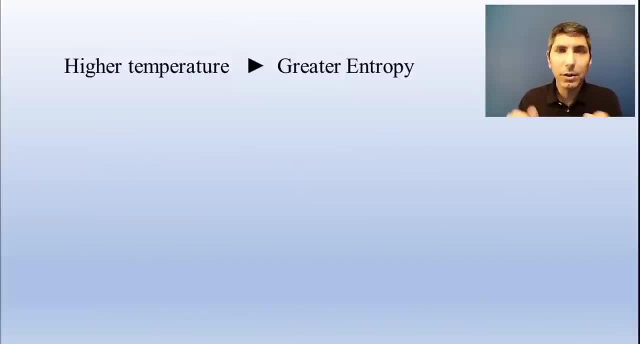 When you raise the temperature of a material, its molecules move faster, so that's more entropy as well. When you increase the volume for a gas, the molecules have more space to move around, so that's more entropy too In this chemical reaction we're going from. 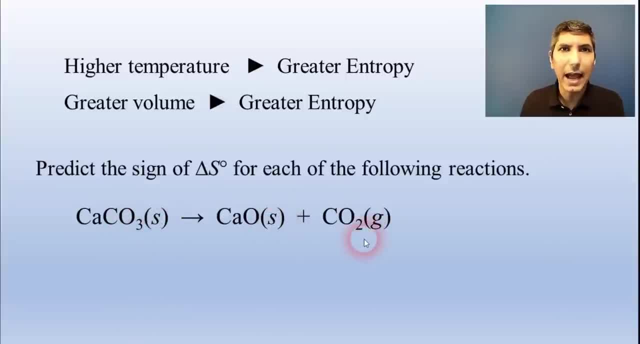 all the molecules in a system to all the molecules in a system. So we're going from all the molecules in a system to all the molecules in a system. So we're going from all solid to a mix of solid and gas. So that's an increase in entropy In a chemical reaction. 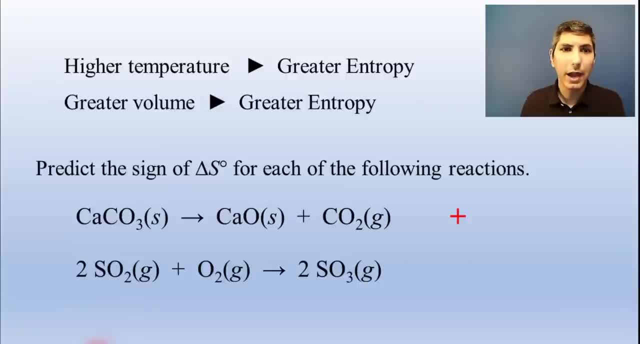 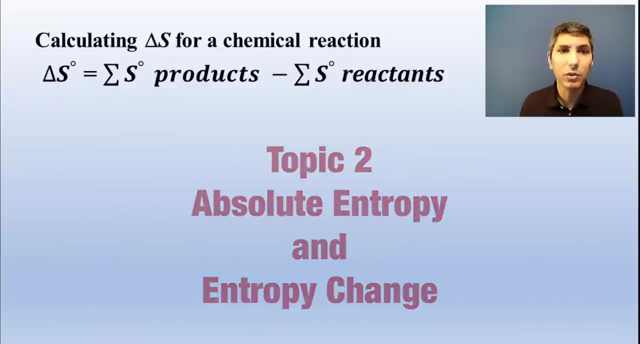 where every substance is a gas. the more molecules you have, the more entropy there is. So if you go from three molecules of a gas down to two, that's a decrease in entropy. We can calculate the entropy of a reaction from the individual entropy values of the substances in the reaction. 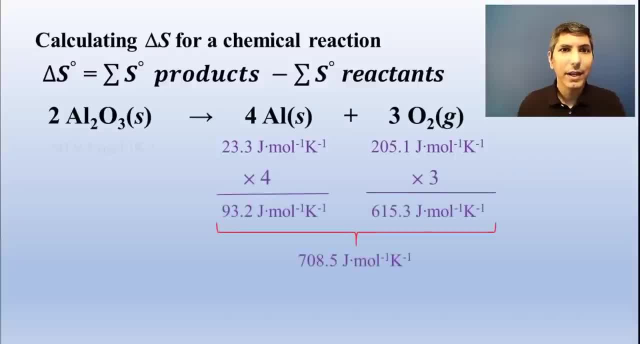 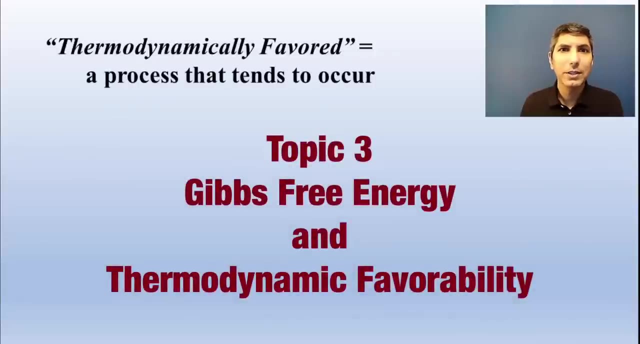 Take the sum of the entropies of the products and subtract the sum of the entropies of the reactants. This is basically identical to the process for calculating change in enthalpy, though we did back in Unit 6.. When a process tends to occur, we say it's. 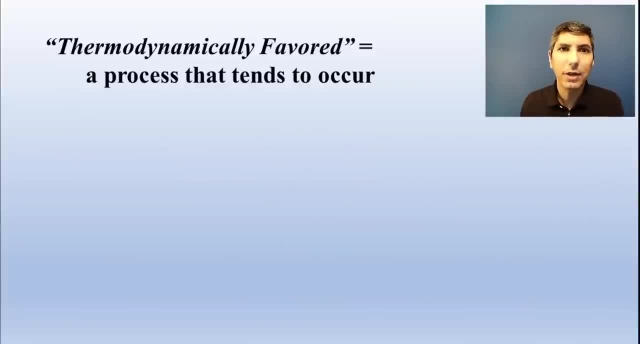 thermodynamically favored. Gibbs. free energy is a measure of the thermodynamic favorability of a process. When delta-g is negative, it's a thermodynamically favored process. When delta-g is positive, it's not favored. Delta-g, as well as delta-s and delta-h, are usually calculated at standard conditions. 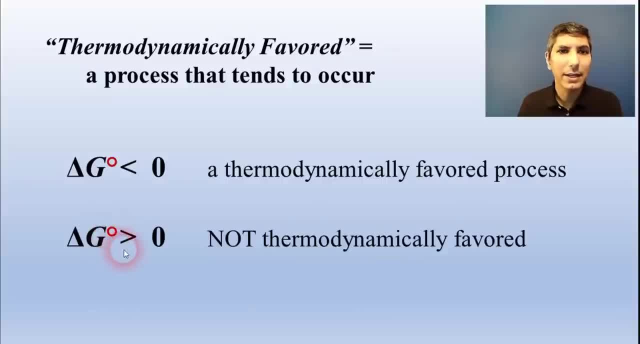 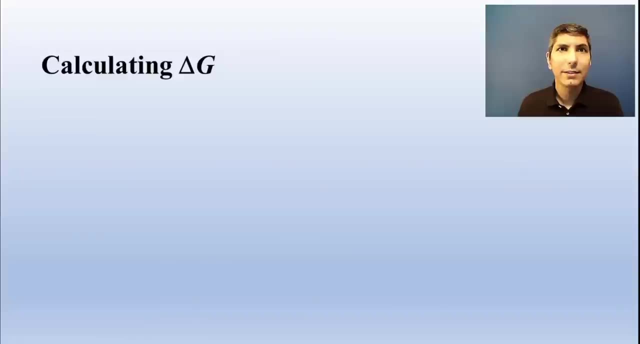 symbolized with this little degree sign. That degree sign tells us that the process is at 25 degrees Celsius, 1 atmosphere pressure and 1 mole per liter for any solutions. There are several ways to calculate delta-g. One way is to take the total sum of the individual. 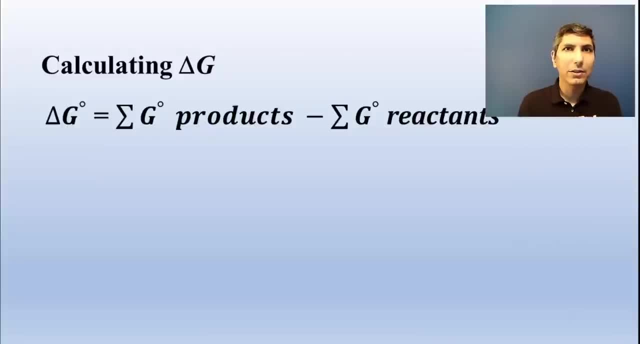 Gibbs free energies of the products and to subtract the total sum of the Gibbs free energies of the reactants, just like we've done previously for delta-h and delta-s, Another way is to use the equation: delta-g equals delta-h minus the Kelvin temperature times delta-s. In fact, 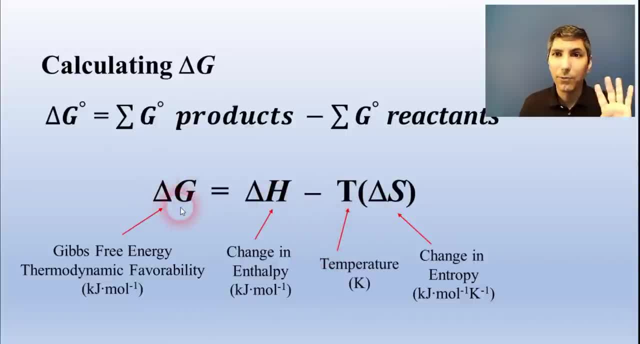 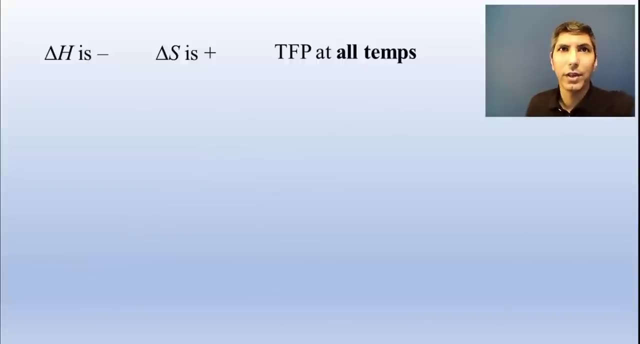 if we know any three of these values, we can calculate the fourth. Just be careful with your units, because entropy is usually given in joules and the others are usually given in kilojoules. The universe tends to favor exothermic reactions, which 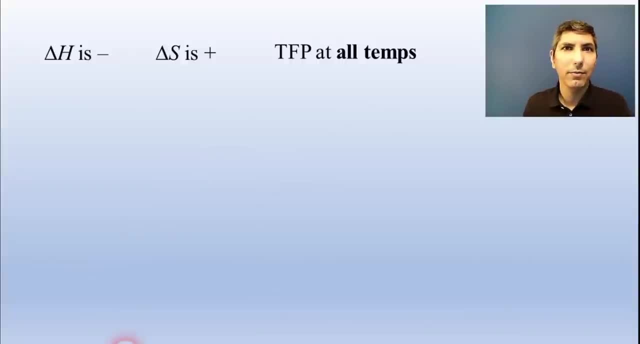 have negative values of delta-h. The universe also tends to favor reactions where entropy is increasing, which has a positive value for delta-s. So if you encounter a reaction that meets both of those conditions, then it will be thermodynamically favored at all temperatures. On the other hand, if a reaction is both endothermic, 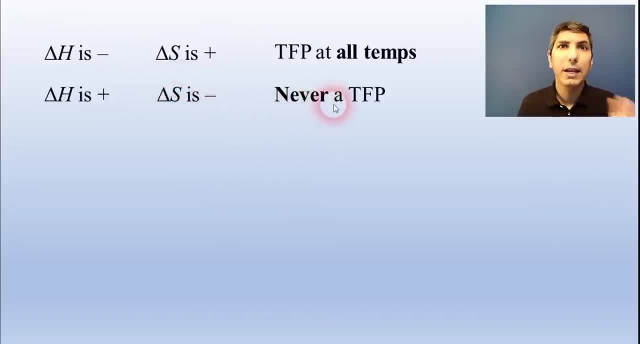 and decreasing in entropy, then it won't be favored at any temperature. If a reaction has a positive delta-h and a positive delta-s, then it will be favored only at very positive temperatures. Likewise, if a reaction has a negative delta-h and a negative delta-s, 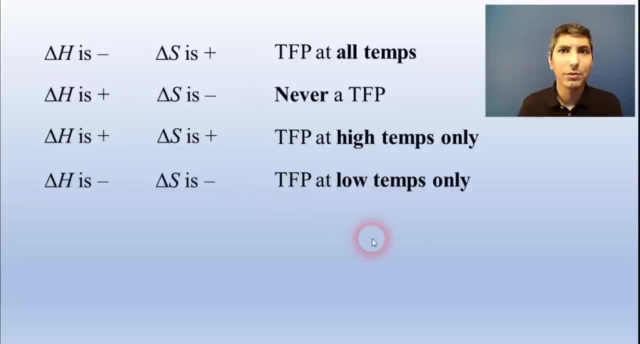 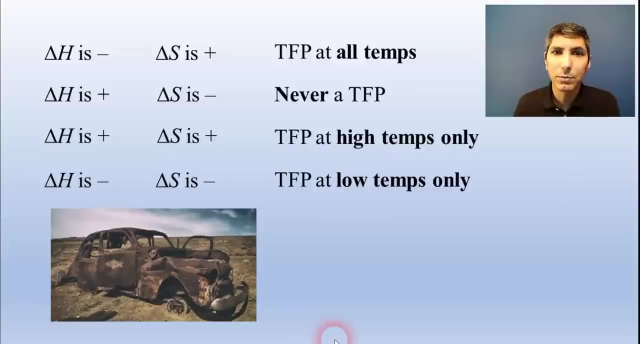 it will be thermodynamically favored at all temperatures. Sometimes you'll encounter a reaction that has an almost immeasurably slow rate, like the rusting of a car. It's pretty much taking place on its own, so we know it's thermodynamically. 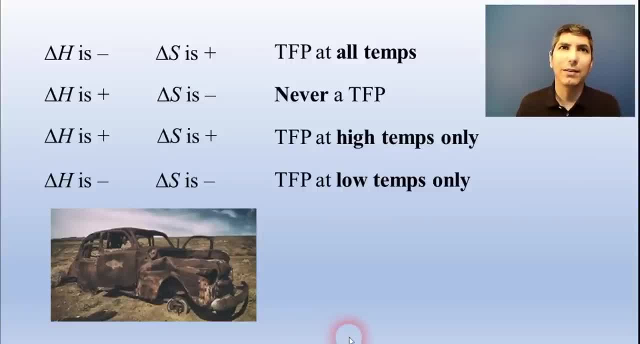 favored, but it's so slow that we can't even measure the rate. This is called being under kinetic control. This usually happens when a reaction has a very high activation energy. It's not at equilibrium and it hasn't stopped. It's just very slow kinetic control. 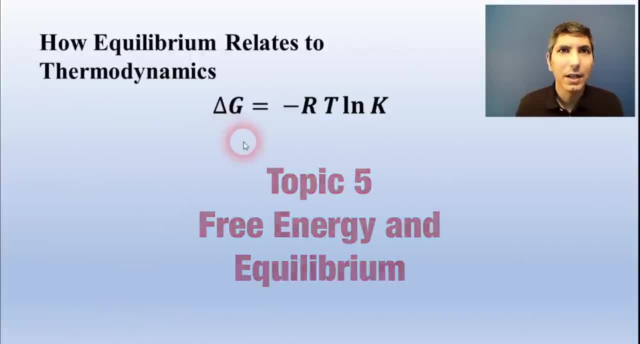 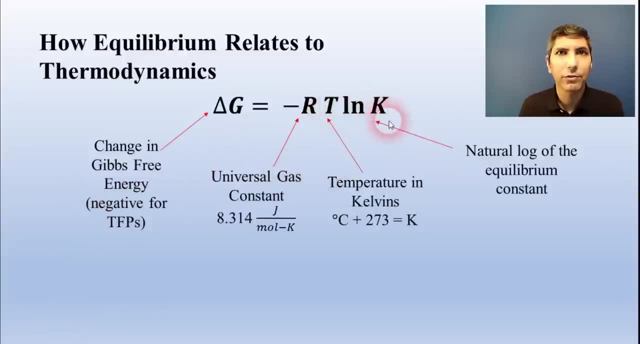 Gibbs, free energy is related to the equilibrium constant by the equation. delta-g equals negative r times the Kelvin temperature times the natural log of the equilibrium constant. where r equals 8.314 joules per mole per Kelvin, We're usually given the temperature. so if we know either 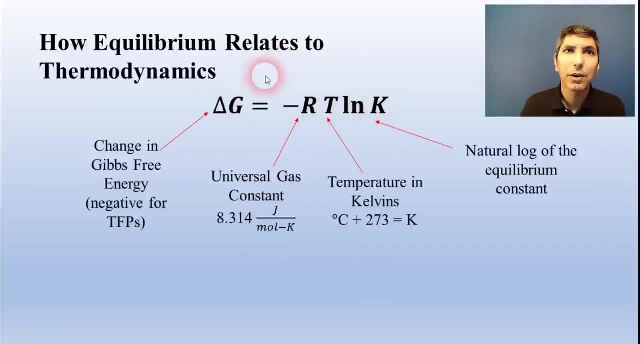 the delta-g or the equilibrium constant. we'll know that delta-g equals a negative r times For the equilibrium constant. we can calculate the other one quite easily Now. this equation tells us that when a reaction is thermodynamically favored, its delta G 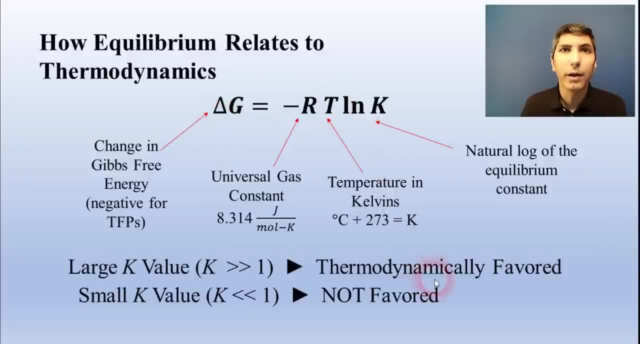 is negative and its equilibrium constant will be a very large number, so will have a lot of product formed. Likewise, when a reaction is not favored, its equilibrium constant will be a very small number, as in much less than one, so almost no products will form. 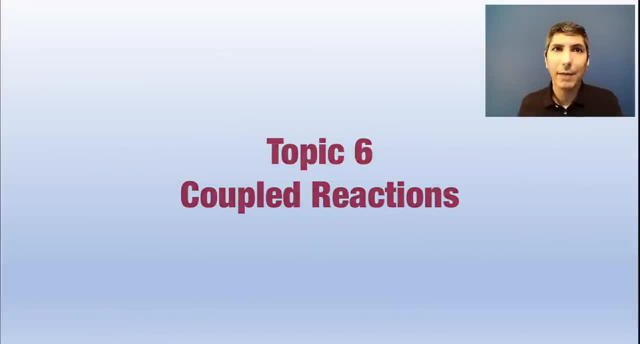 Some reactions that are thermodynamically unfavorable can still happen. We might have to add external energy like electricity or even light. This is how you charge a cell phone battery or get carbon dioxide to react with water in photosynthesis. Another way is to couple the unfavorable reaction with a more favorable one. 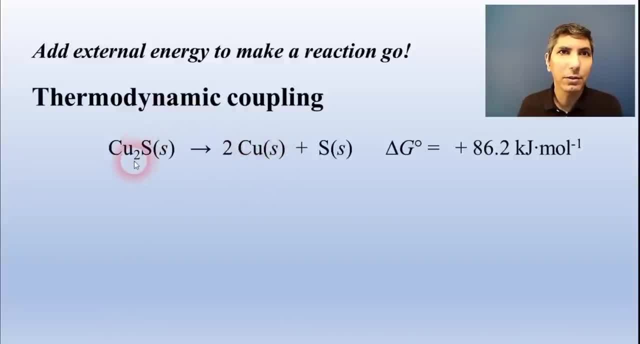 For example, obtaining copper metal from copper sulfide by itself probably isn't going to happen because the delta G is positive, it's unfavorable. But if we throw in this equation that is favorable and we add them together, we see that we just 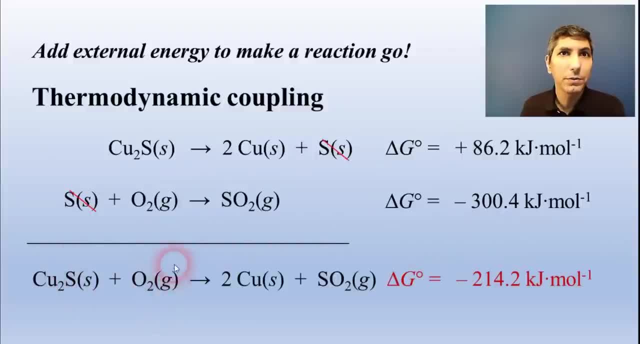 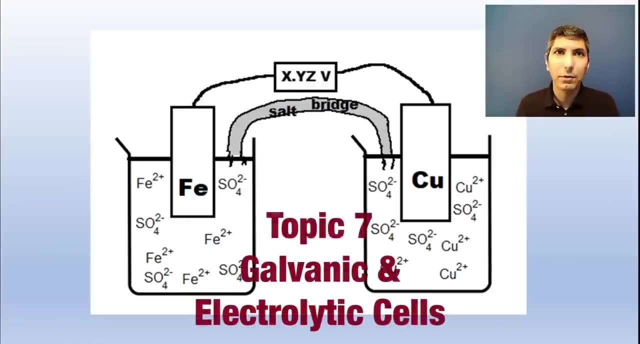 need to react the copper sulfide with oxygen in order to obtain copper from copper sulfide to have a process with a negative delta G. A galvanic cell is what most people call a battery. It's thermodynamically favored. It basically uses wires and electrodes to harness the electron flow of a redox reaction. 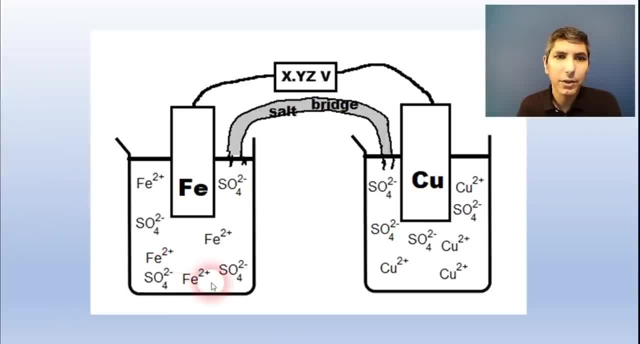 to power a load. We use a diagram like this to visualize what's going on in the galvanic cell. Each side of the cell has one specific half reaction that's taking place. The side where oxidation takes place is called the anode. 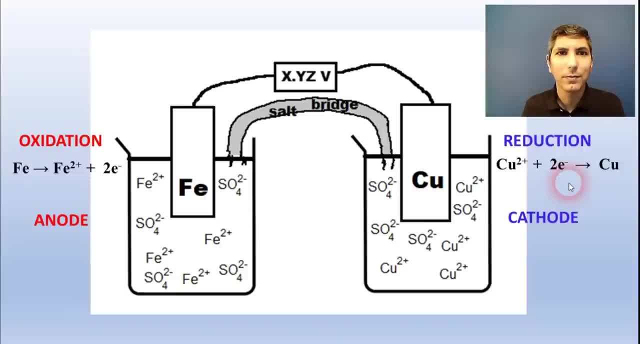 And the side where reduction takes place is called the anode. Remember that the electrons flow through the wire from the anode to the cathode, like AC. If these are metallic electrodes, the cathode should always increase in mass. The cat gets fat. 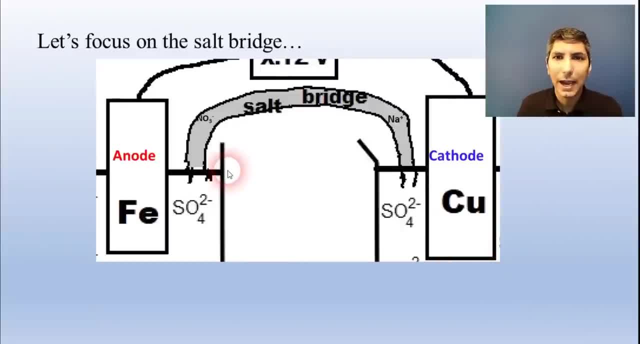 The salt bridge equalizes the charge as ions react at the electrodes For the salt bridge. we use ions that won't react at the electrodes For the salt bridge. we use ions that won't react at the electrodes But won't react with anything else in the galvanic cell. 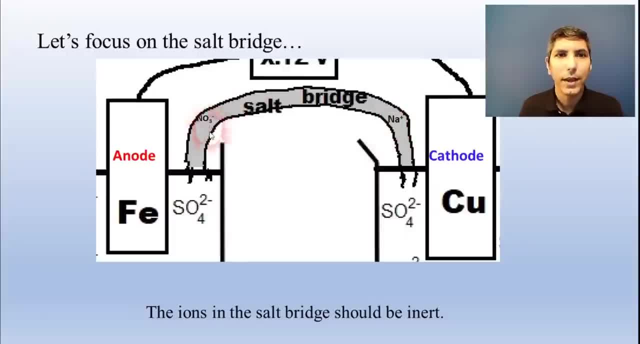 So sodium and nitrate ions are common choices. At the edge of the salt bridge, cations flow toward the cathode And anions flow toward the anode. You can use the clues given to you in the question to figure out every one of the other. 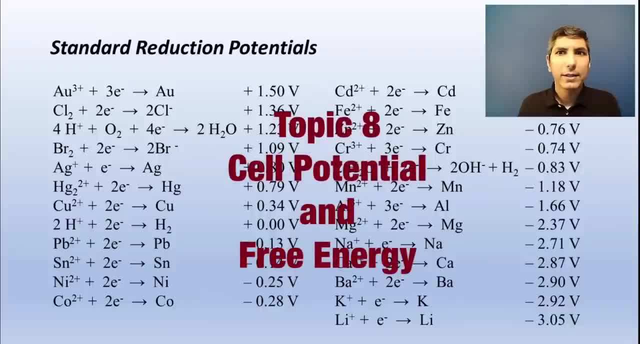 details about the galvanic cell. Every galvanic cell has a cell potential, sometimes called its voltage or its potential difference. In our list of half reactions, notice that these are all written as reduction potentials, even though every redox reaction has one oxidation and one reduction. 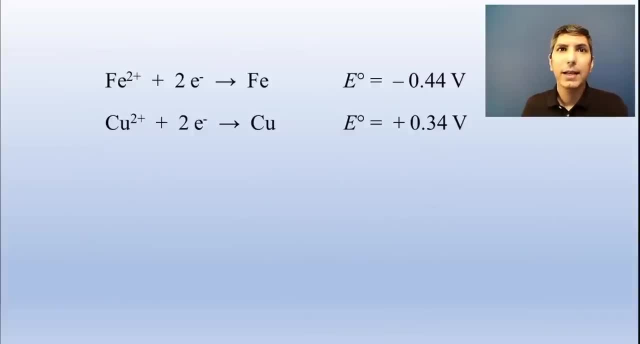 We use these standard reduction potentials as written and calculate our cell potential by taking the value for the cathode from the list and subtracting the value for the anode. The cell potential is related to the thermodynamic favorites. Here we have cations flowing in anode, then cations flowing in a nào potential and anode. 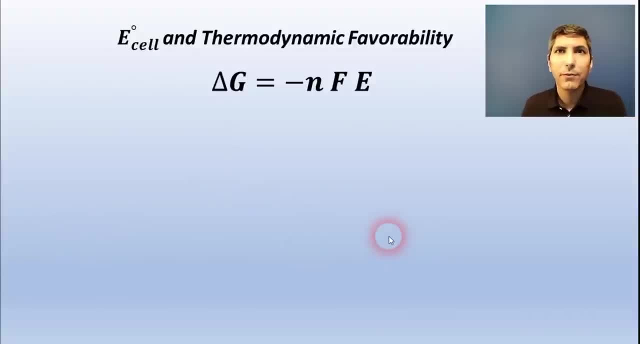 We canarat is aчеых and cation Bеqpcten, Bеqpcten mode. dynamic favorability of the cell. by this equation, The delta G of the cell equals the opposite of the number of moles of electrons transferred in the balanced equation times. 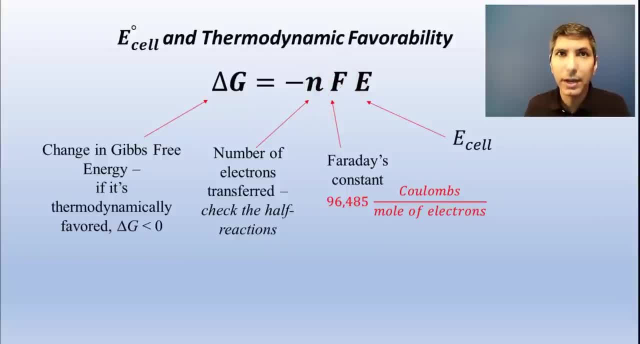 Faraday's constant, which is 96,485 coulombs per mole of electrons, times the cell potential. We can determine the N by balancing the equation. So if we know the delta G or the cell potential, we can calculate the other one. Cells with a positive voltage are thermodynamically favored. 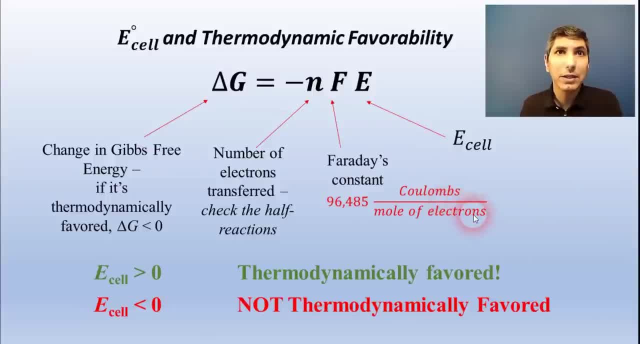 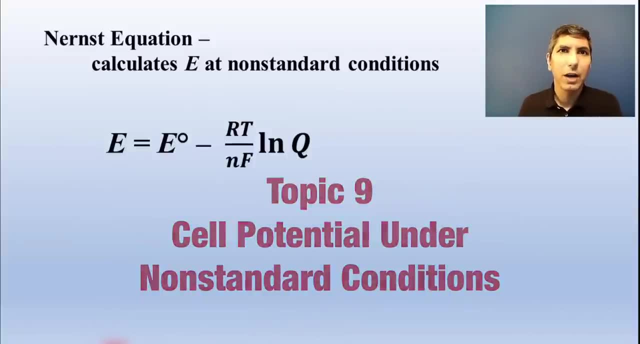 while cells with negative voltage are unfavored and would need some external power source. We normally calculate cell potentials at standard conditions which honestly, aren't that common in the real world. For non-standard conditions we use the Nernst equation. Now some of these values. 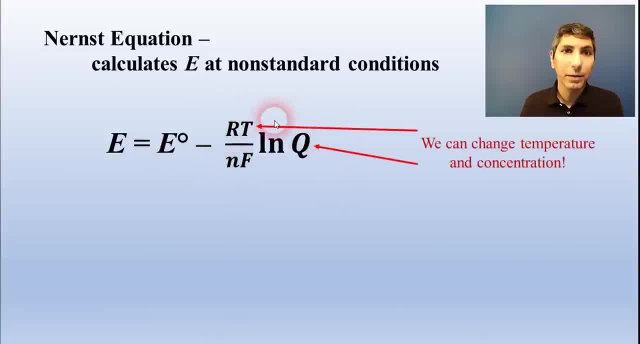 don't change in a reaction, but we can change the Nernst equation So we can calculate the temperature and concentration. If we increase the concentration of the products or decrease the reactants, that increases the reaction quotient Q and that lowers the voltage. Conversely,